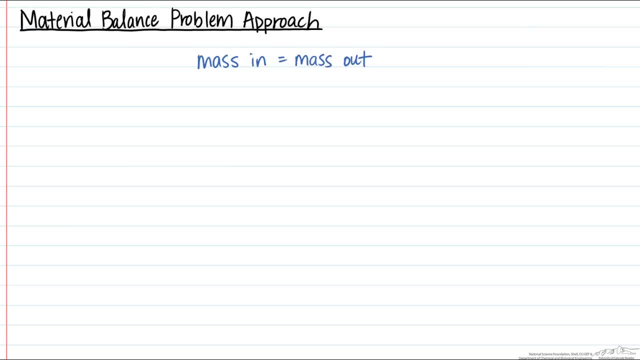 what does the problem ask for? Write it in terms of variables that you set. Read the problem carefully. Ask yourself: what do they want? Look for key words or phrases. If you see something like overhead product, then it means that you have product coming out. 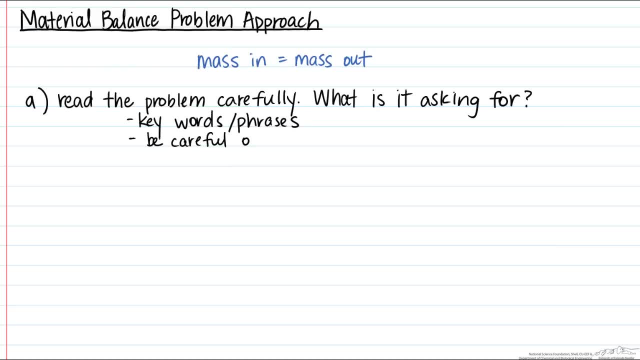 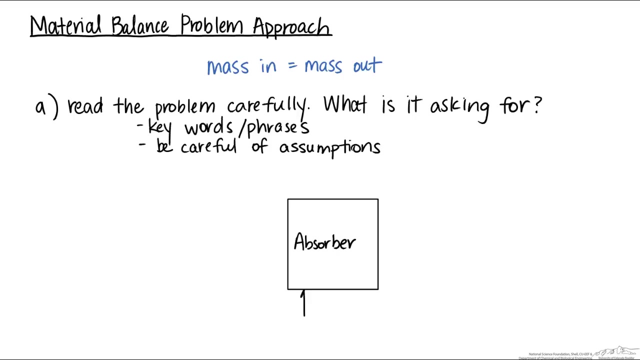 of the top of, perhaps, your column. Be careful of what you assume. Some examples of this are adding streams, leaving streams out, and let me show you a typical example. Let's say we have an absorber, There's a gas stream that comes in and comes out, And a pure liquid. 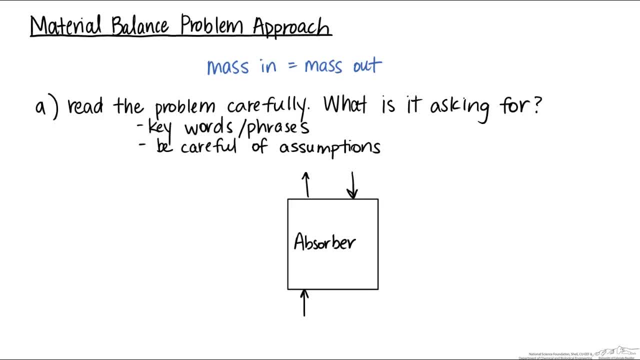 enters the absorber to absorb some of the components of the gas stream. Well, if this stream enters the system, it needs to exit the system. even if the problem doesn't specifically say that there's an aqueous stream exiting the system, It has to come out even if it's. 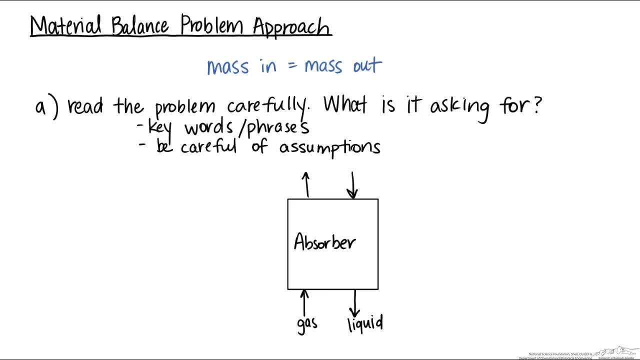 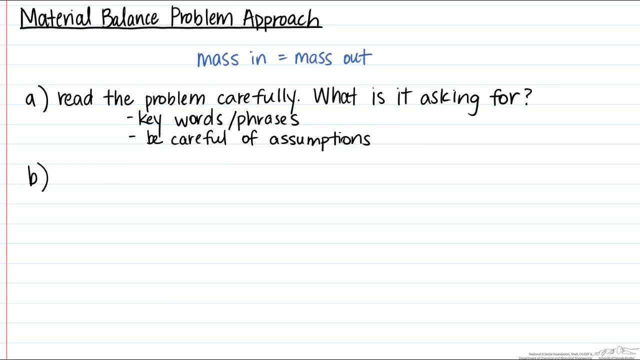 not pure. in fact it probably isn't, because the purpose is for it to pick up some of the components from the gas stream. The next thing to do is draw the picture, Label the unknowns and the knowns. What I tend to do is I use m for mass and I use n for moles. For simpler problems, I'll use x. for our mass fractions. M1 is the number of moles. M2 is the number of moles. M3 is the number of moles. M4 is the number of moles. M5 is the number of moles. M6 is the number of moles. M7 is the number. 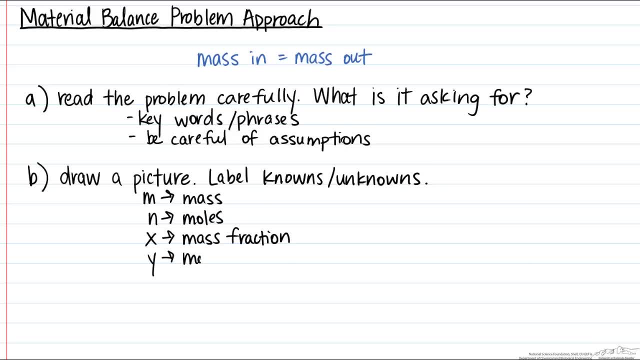 of moles. If I'm looking for a particular mass fraction or mole fraction, I tend to label it with something that indicates the component. So, for example, if I have a mass fraction of benzene, I'll call this x sub B. Finally, if there is more than one stream that has benzene, let's say there is. 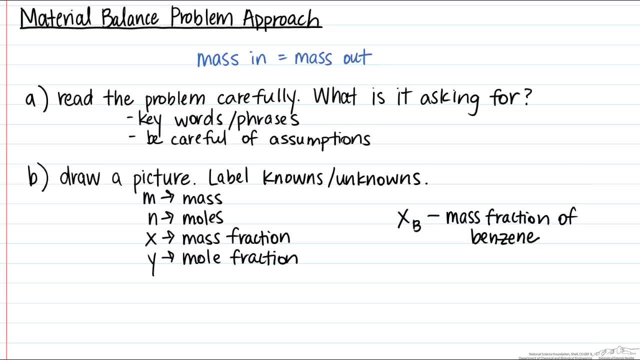 benzene in stream 2 and in stream 4, I'll write X sub B2.. The more organized you are, the easier it is for you to solve. Another suggestion is to solve for the easy unknowns ahead of time. Don't do major calculations because first of all, you may end up confusing. 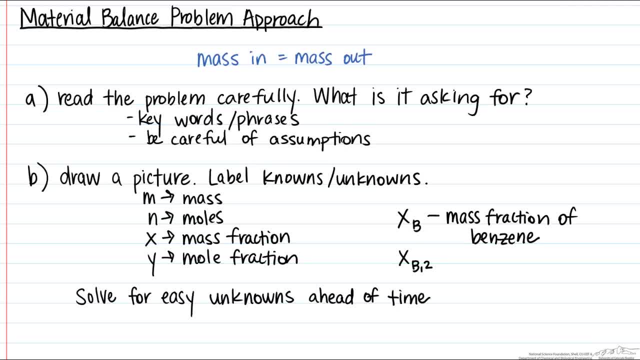 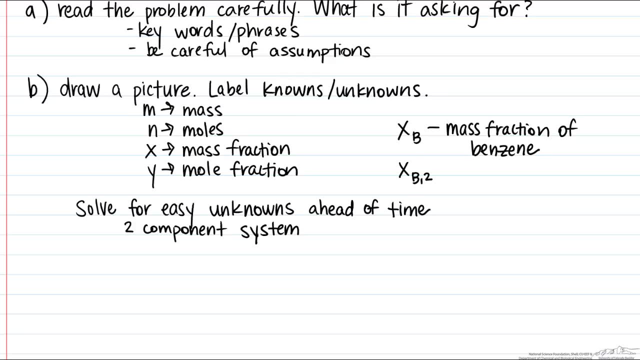 yourself. and, second of all, somebody looking at your flow chart may not understand how you got a certain number, But things like: if you have a 2 component system and it says that it has a mole fraction or 40% benzene in stream 4, then you're going to have a 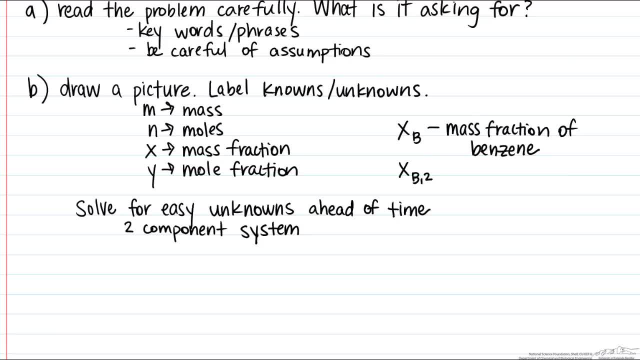 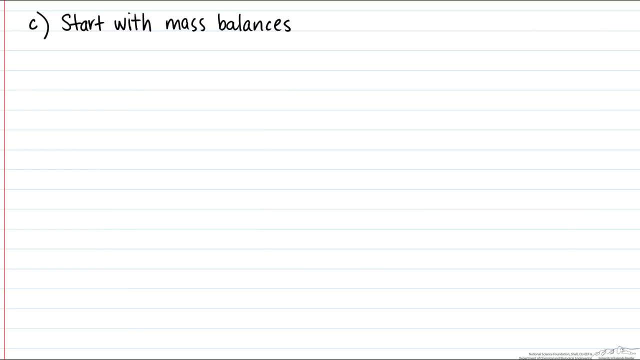 total of 20,000.. And that's equal to 40. So it's not m base times the total of 20,000, but it's a total of the total channel at which you're going to have a mole fraction. Now we can write 0.60 benzene and the rest toluene. You can write 0.40 benzene and 0.60. 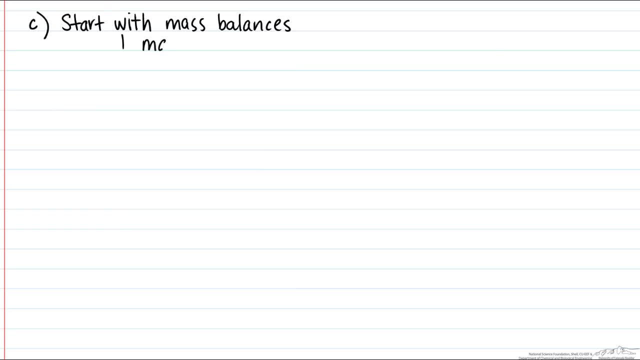 toluene. Now we start with the material balances, And the thing to remember is that there is one mass balance for every component. One thing that you can do is take your desequation and you can write it down again, And that's a memento, So you can write down the number. 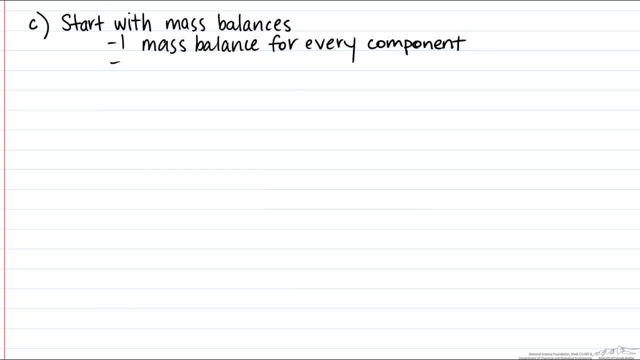 do is that you can substitute one overall balance for a component balance, And one of the things that you have to be careful of when you are doing your mass balances that each one of your equations or balances is independent. So let me show you an example. 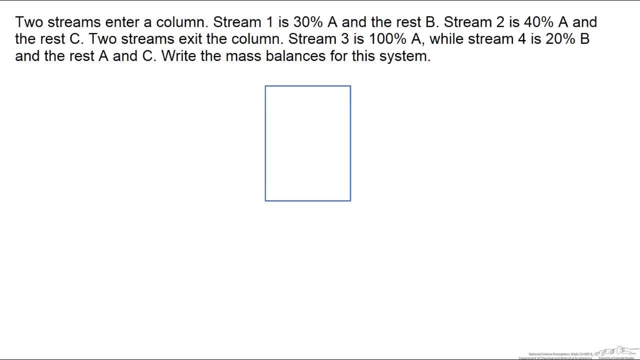 We have two streams that enter a column. Our stream 1 is 30% A and the rest B. There is an example of solving for simple unknowns. Stream 2 is 40% A and the rest C, So two streams exit the column. 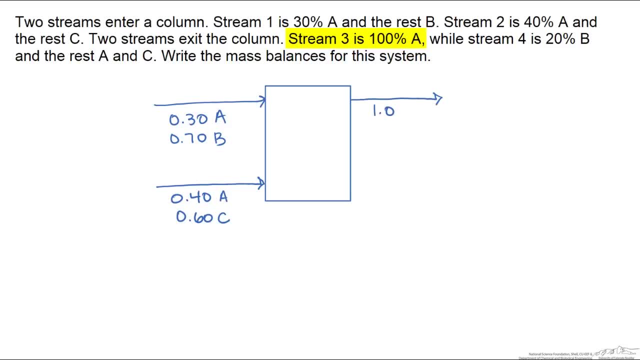 Our stream 3 is 100% A and stream 4 is 20% B and the rest A and C, And we are going to write this using the fact that the sum of the mole fractions equals 1, so our x sub c is equal to 0.8.. 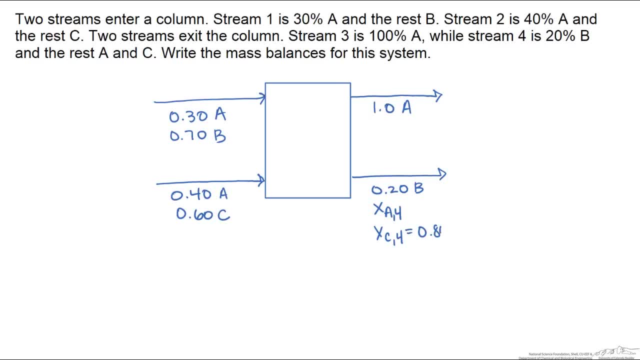 0.8.. 8 minus x sub a, And we're going to assume that everything is in mass fractions, And so we need to write the mass or material balances. We'll call this m1,, m2, m3, and m4.. So now 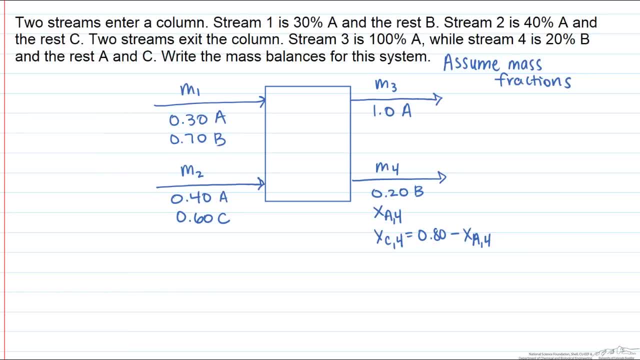 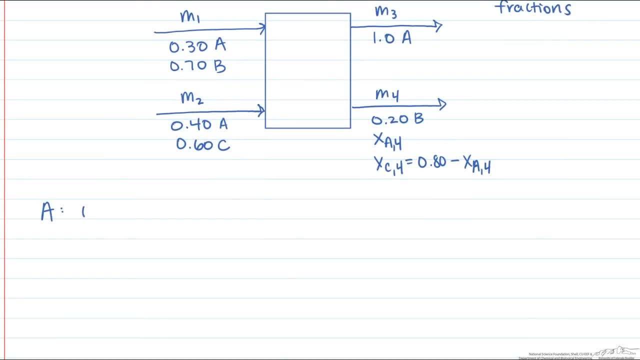 let's do these mass balances And we'll start with a. The amount of a that comes in is 30% of m1 plus 40% of m2. And exiting we have 100% of m3, or just m3, plus our x sub a times. 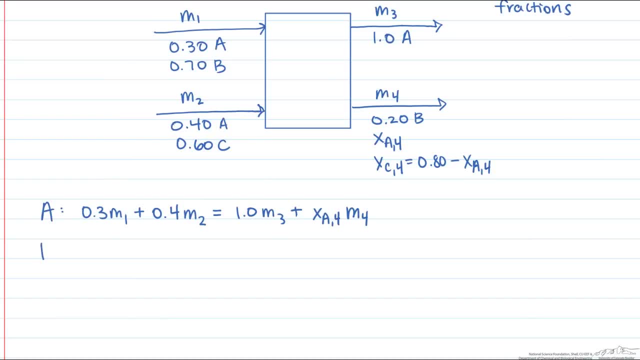 m. And here we have m to d, x to the power 3, and we're going to presented with a non-elemental fraction of f minus a per front line, z star. And then we'll see that because the mass balances M4.. Now we'll do the B balance Coming in the first stream, 70% is M1.. There's nothing. 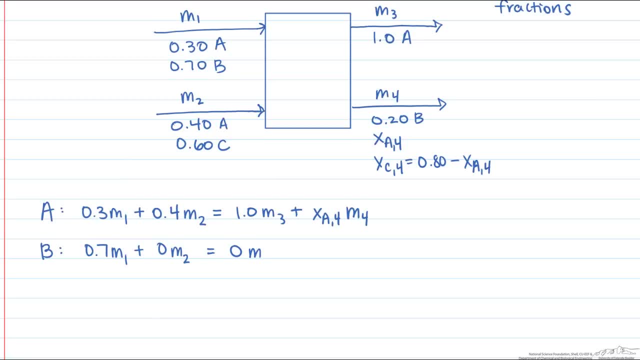 in M2.. There's nothing in M3. It's 20% of M4.. Now our C balance, which nothing is in M1. C is 60% of M2. And coming out we have 0.8 minus x sub a. 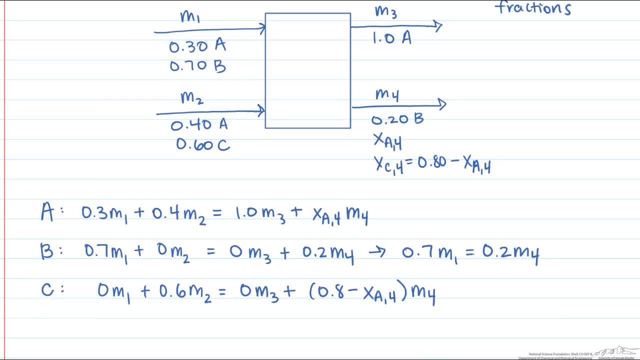 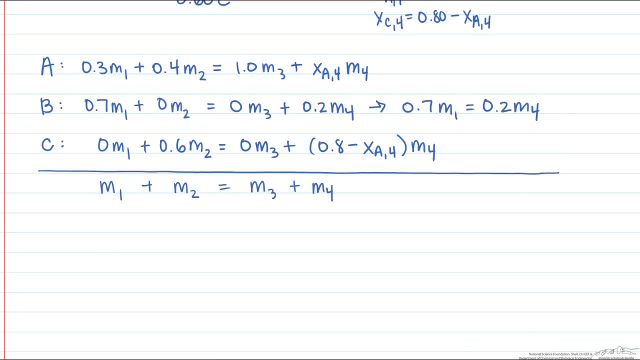 Times our M4.. These are our three component balances. Let's see what happens if we add them all together. So note: when we add them all together, what we get is the overall balance. So we can only use three out of these four equations to solve our system.